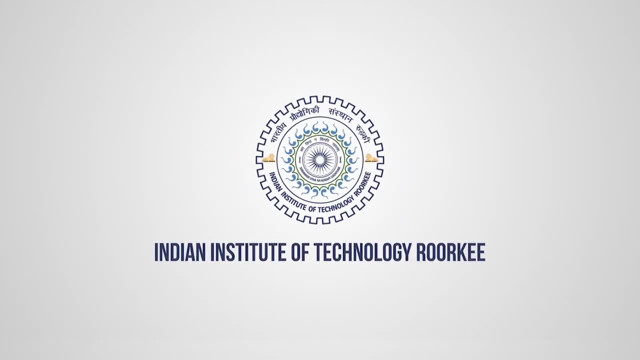 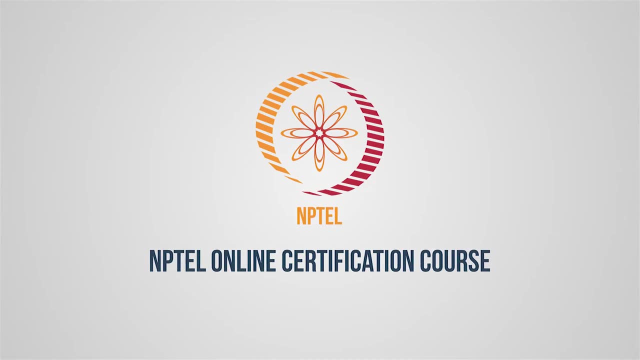 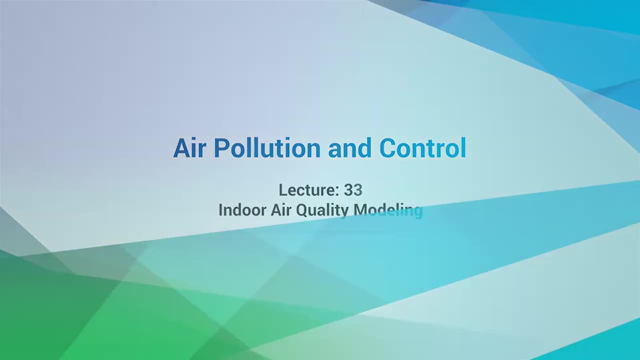 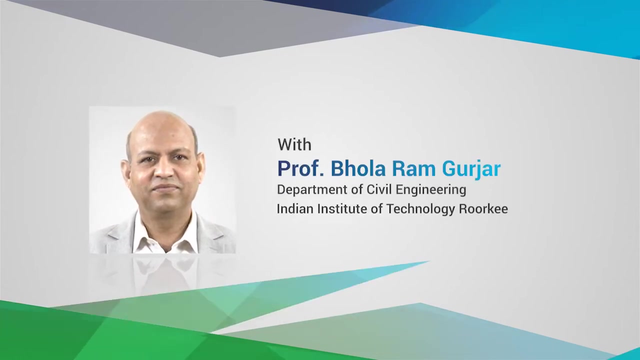 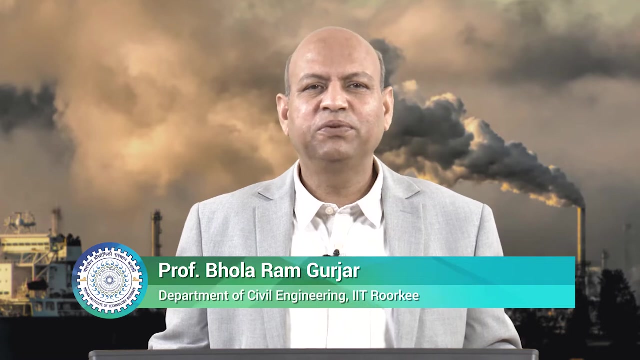 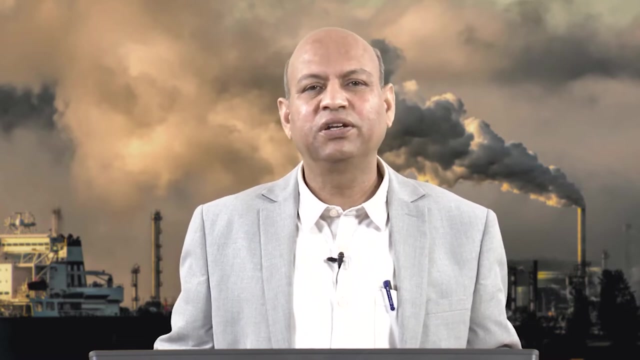 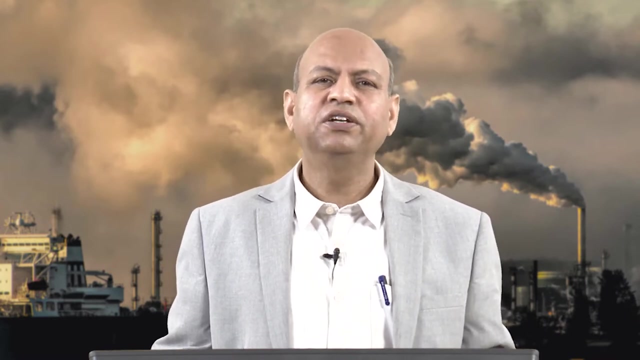 Hello friends, you may recall we discussed, you know, at certain point of time about ambient air quality modeling, like Gaussian dispersion model and so on. Today we will discuss about indoor air quality modeling. How do we model the indoor air quality? Because just before this lecture we have already discussed about 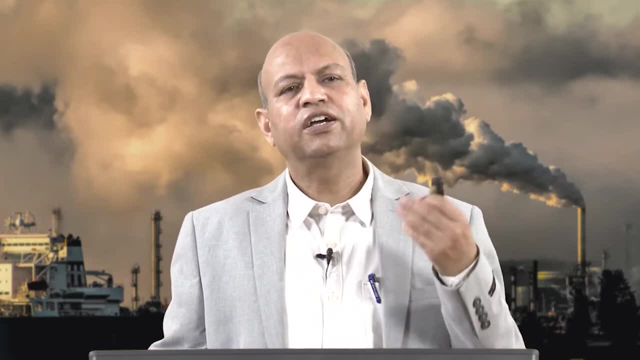 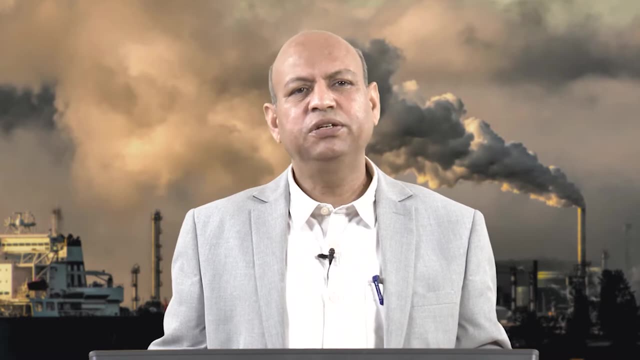 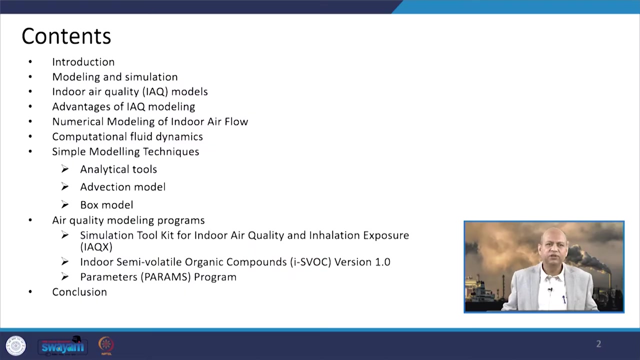 various sources of the indoor air pollution and then exposure assessment through monitoring, sampling of the indoor air quality or indoor air pollution. So today we will discuss how to model or simulate the indoor air quality. This will include introductory part and then what are the modeling and simulation? How do we relate these modeling issues and simulation? 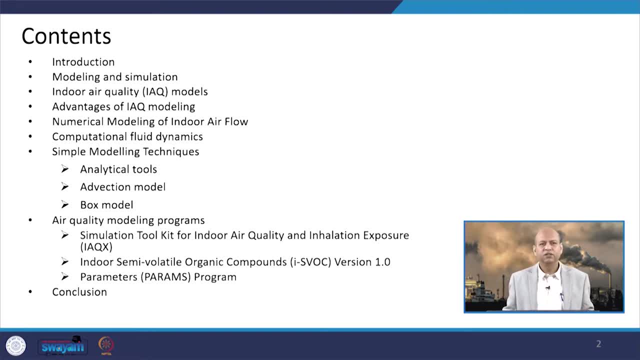 aspects of mathematical modeling when we do about the indoor air pollution, Then indoor air quality related models. very, you know, simple models. those kind of models we will discuss Analysis of the modeling means with respect to like monitoring or sampling. Then numerical modeling of air flow. indoor air flow we will look into. Then computational fluid dynamics. 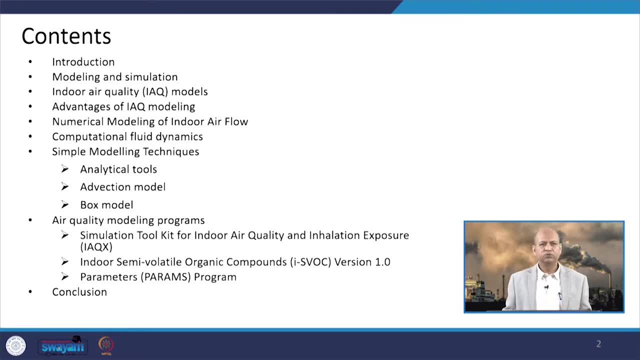 related important aspects which are, you know, used for indoor air flow or modeling, So that we will discuss Then simple modeling tools or techniques, like analytical tools and advection model or box model, which are quite popular For modeling indoor air quality, so that we will touch and later we will discuss on air. 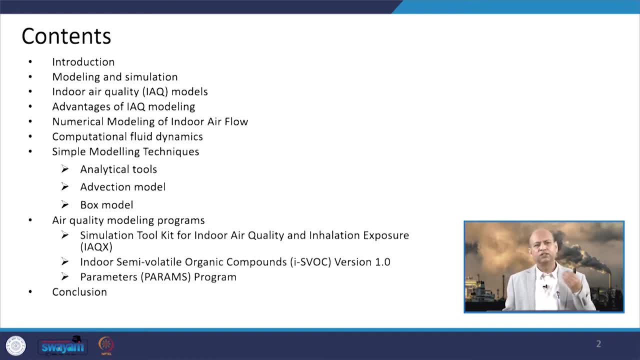 quality modeling programs or tools which are already developed by US EPA, like you know: simulation tool kit for indoor air quality and inhalation exposure that is known as IAQX, and indoor semi volatile organic compounds, IASVOQ, version 1.0.. And then third one is: 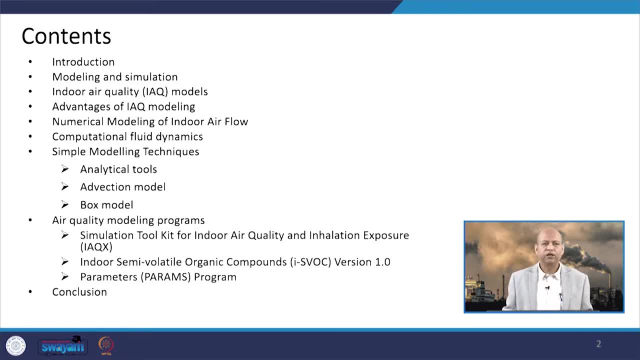 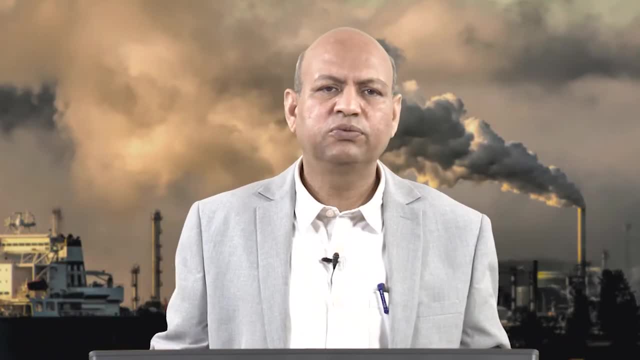 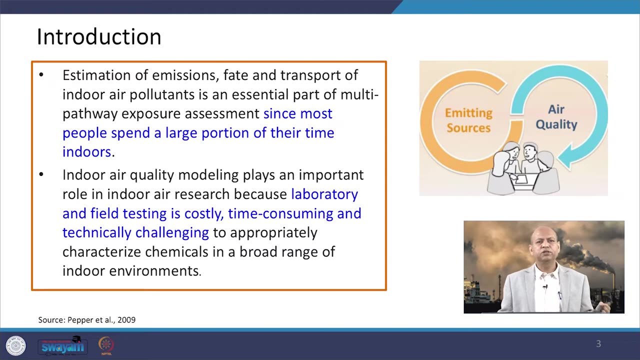 parameters or PARAMS program. These three popular tools, or easy to handle tools, we will discuss which take care of air quality modelling in indoor environments, and then we will conclude. So when we talk about introductory part of indoor air pollution modelling, basically, whatever sources are there, or sinks are there, if we do not consider them to simulate or 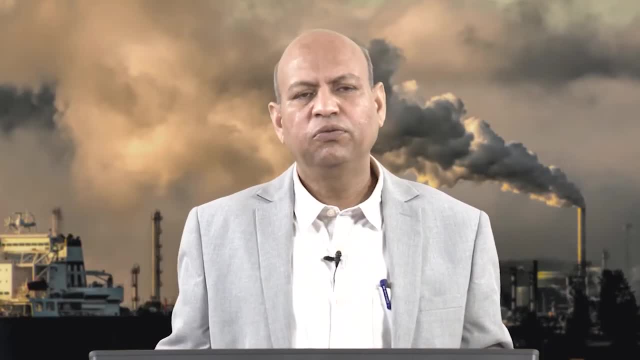 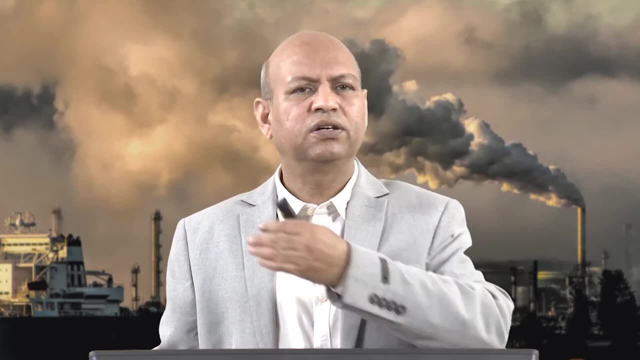 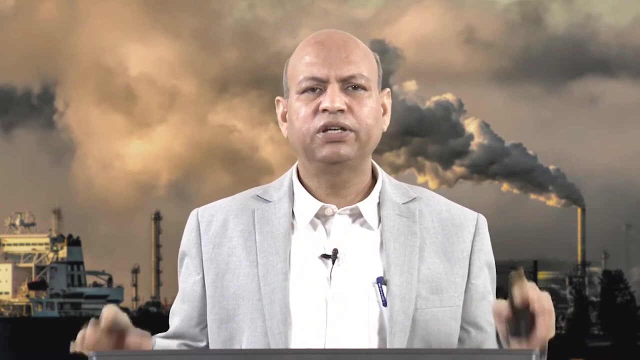 model, then it is difficult to find out how much concentration will be at a particular place And, moreover, if we go for sampling like each and every corner in the indoor environment, then it needs lot of resources and lot of time. So better we have optimum number of samples and, based on the sample data, we can have certain 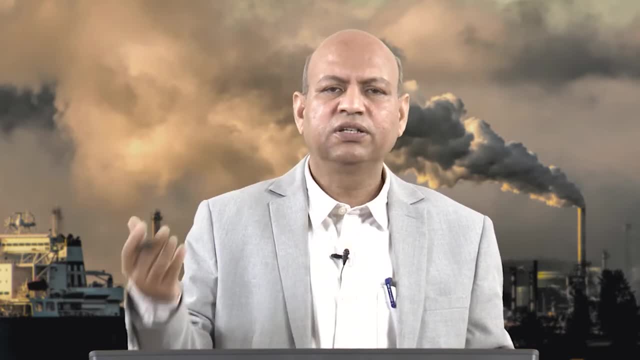 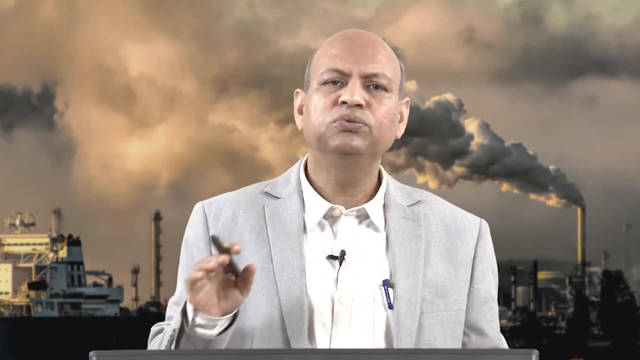 modelling techniques which can be used for taking these results further. So, for example, let us say health risk assessment, etcetera, but before that we need to do the air quality modelling of the indoor environment. only then we would be able to use that further. 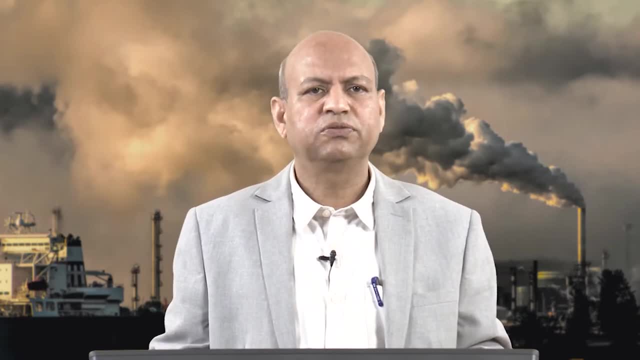 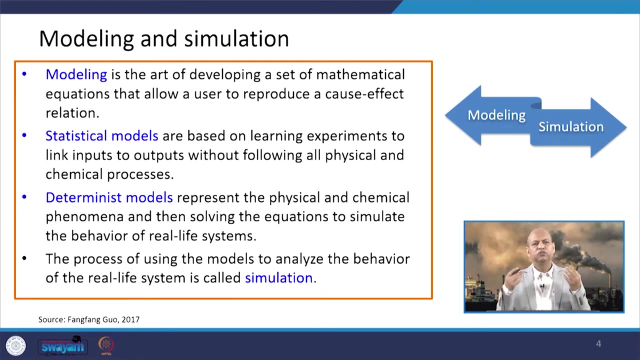 in health risk assessment and those sort of activities. When we talk about modelling and simulation, So modelling as it is nothing but the set of equations which represent the reality of whatever thing we want to model. and there may be different modelling techniques, like models which are used based on certain input output relationship, without giving much importance. 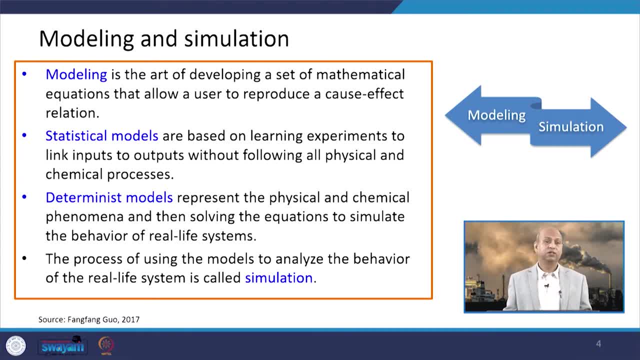 to physicochemical interactions or processes. But there are other modeling techniques, like deterministic models, which take care of physical and chemical phenomena and they solve those physicochemical characteristic related equations. then they get the result. but they are like resource consuming or time consuming and it 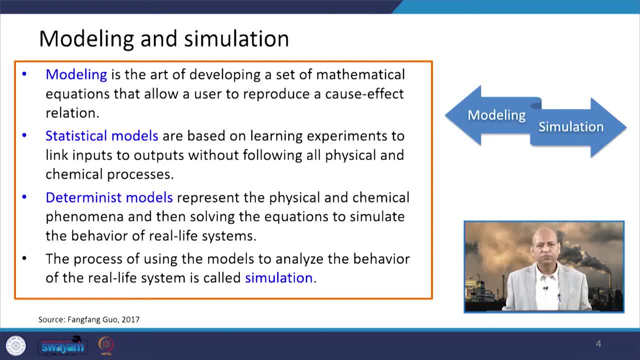 also needs skilled manpower to handle those kind of models. And whenever we process using any sort of model, whether it is a statistical model or deterministic model, whenever we are using a model to process the data and we are analyzing the behavior of any real life system, then we call it as a simulation. we are doing a 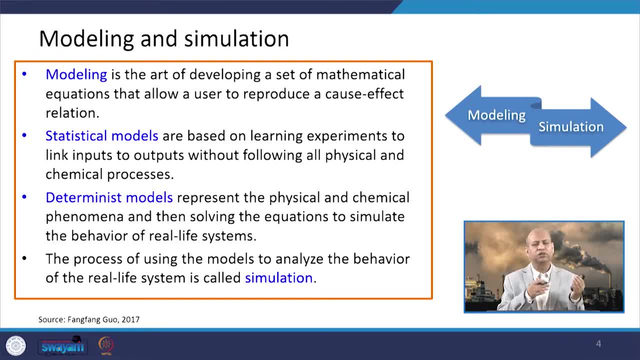 simulation. So whatever, whether it is in ambient air or indoor air or any kind of environment we are talking about And we are trying to use certain model to represent that, those processes which are related to that environment, whether of indoor or outdoor. So we are basically simulating that particular environment of different aspects of that environment. 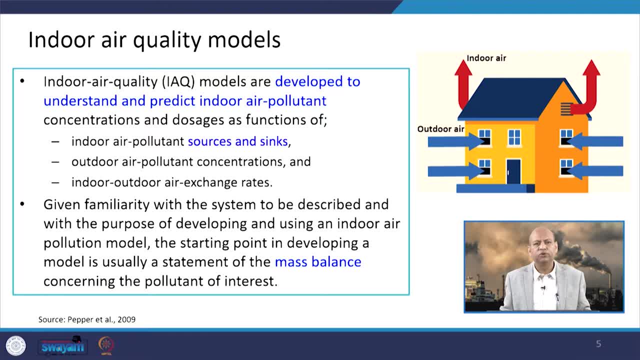 Now, if we talk about indoor air quality models which have been developed to predict or to estimate indoor air pollutant concentrations, and then after that dosage, you can say: because those function is important for exposure assessment and risk assessment. So basically three functional parameters are important to model indoor air environment. 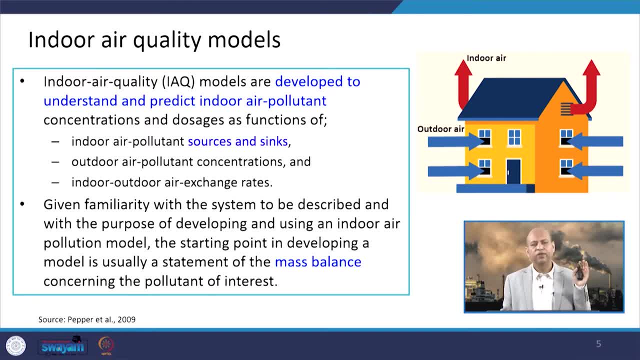 like indoor air pollutant sources and sinks. we should know about what are the different sources of those indoor air pollutants and what are sinks also, because some portions will be like absorbed or adsorbed. those kind of sinking related phenomena will also be there. And outdoor air pollutant concentration we should also know the reason is because outdoor 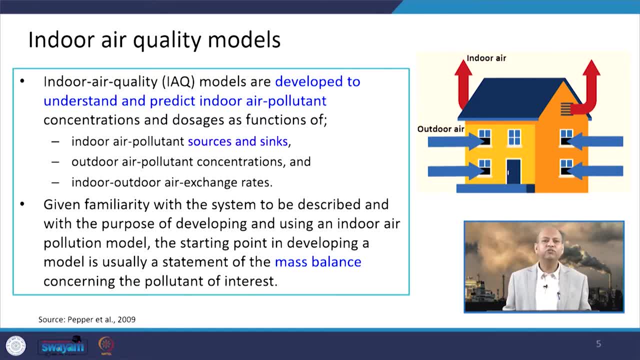 air pollution also come to the indoor environment through like windows, through other doors whenever we open. So the concentration outside will also influence the indoor environment. like this, outdoor air can enter into the inside of the house. So we need to know how much ambient air concentration is there and also the indoor outdoor air exchange. 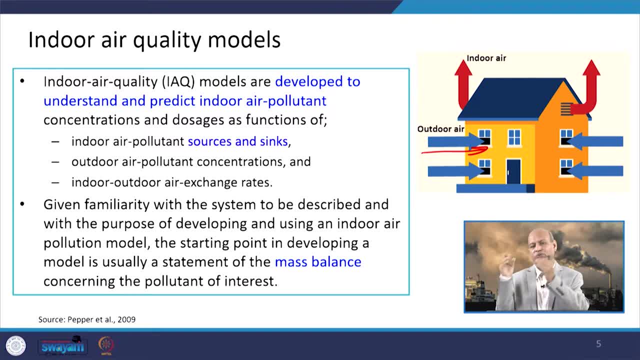 rates Because they will interact: indoor environment and outdoor environment. they will interact whenever like door is opened, window is opened or any other system we are using. So those air exchange rates we should know about Now, like we know this system, which is described in the form of developing or using an indoor 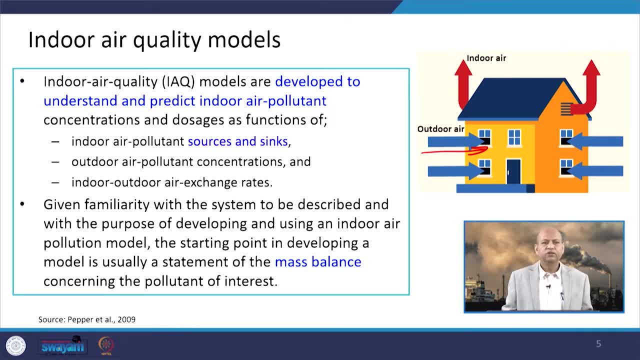 air quality model or indoor air pollution model. So we need to begin with, So let us see, So let us see, So let us see the, So let us see the certain principles and the mass balance concerning those pollutants. 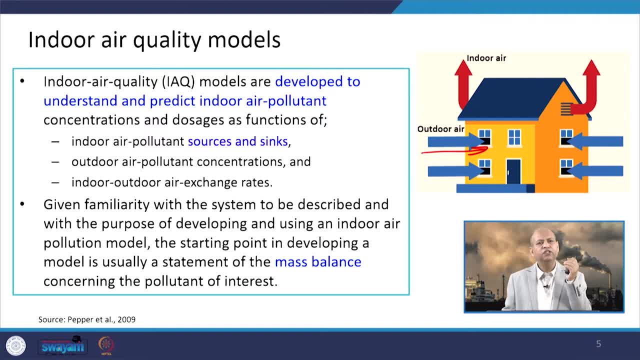 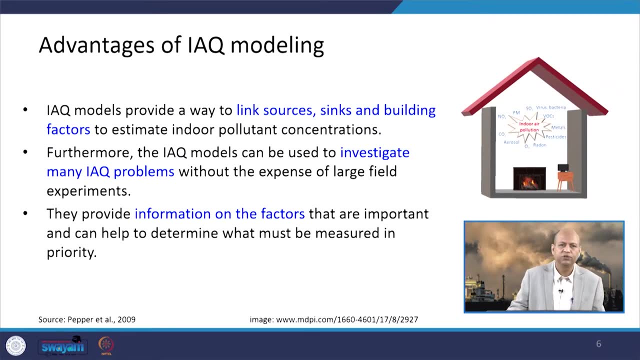 which are of our interest in the indoor environment. basically we look into that. So you might have heard about like mass conservation or energy conservation. So from that perspective, mass balance related equations we use in this particular indoor air quality modeling efforts And what are the advantages? 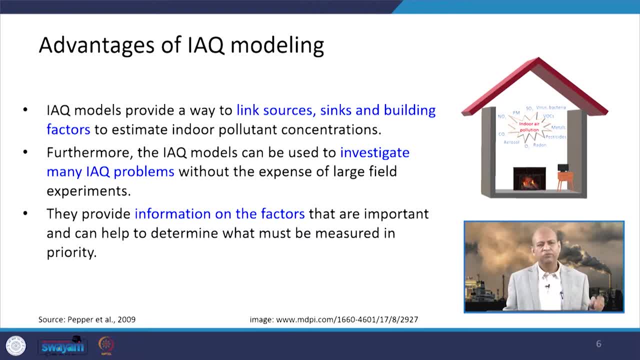 Why do we do this indoor air quality modeling, Although we have touched upon like- because we cannot go for monitoring or sampling each and every corner of the environment and it needs lot of resources. So one advantage is that whenever you have a valid model so you can run it and get the 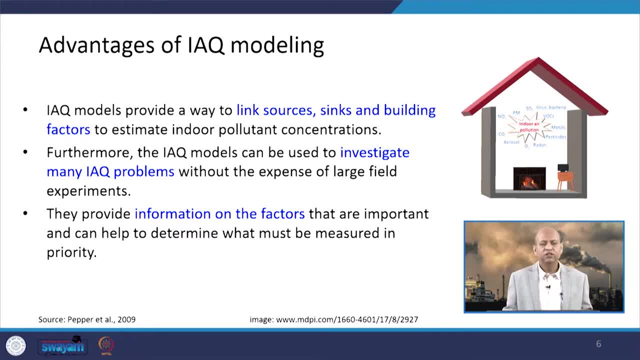 concentration with respect to different scenarios. So it provides basically the way or understanding to link the sources and sinks and the building factors. building factors, like which influences the air exchange rate, as I said, like outdoor environment, indoor environment, are interacting through those windows and doors. 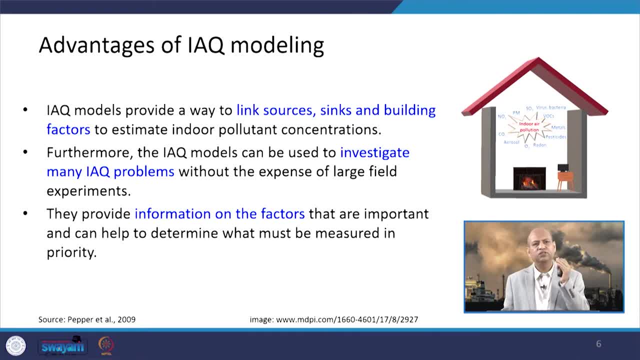 So those factors, building factors, they influence. so these kind of parameters or variables are linked through that modeling effort. Then also it is used for investigating many IAQ or indoor air quality related problems, without any additional expenses which are required for field activities. 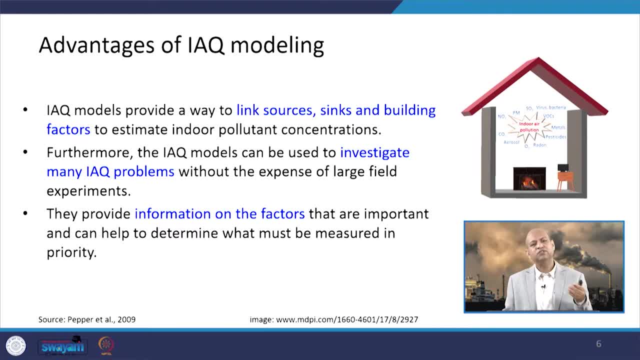 Field experiment. let us say so. we can avoid field experiment. we can just create a scenario and with respect to that scenario, we can get or predict certain concentrations and we can know that this will be the effect of the changes if you want to make in the indoor. 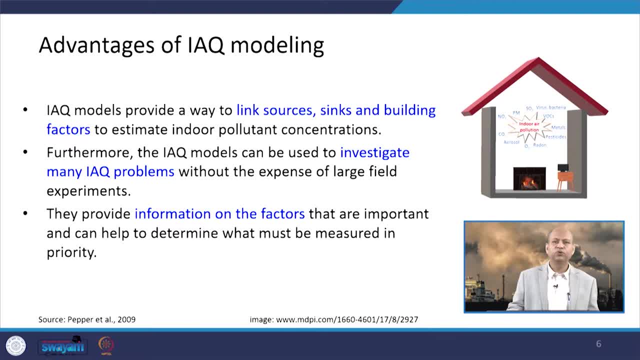 environment. Suppose we want to go for some other energy system, like heating system in the indoor environment, whether it will influence the air quality or not, or we are going for another kind of project And furnitures also have certain sources of these VOCs, et cetera. 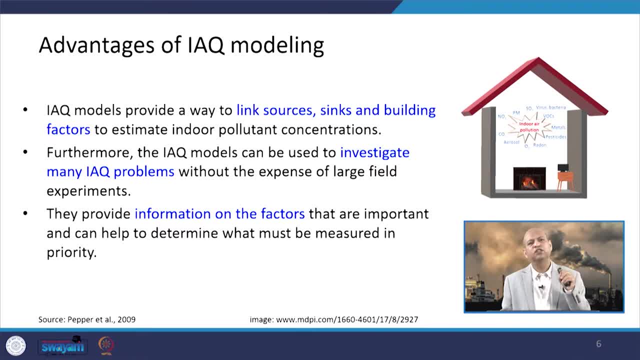 So those variables can be there and those variables can easily be simulated in the modeling technique. They also provide information about the factors which are very important and they determine the indoor environment related issues, whether not only the like air quality is the final result, but before that there are many variable factors. 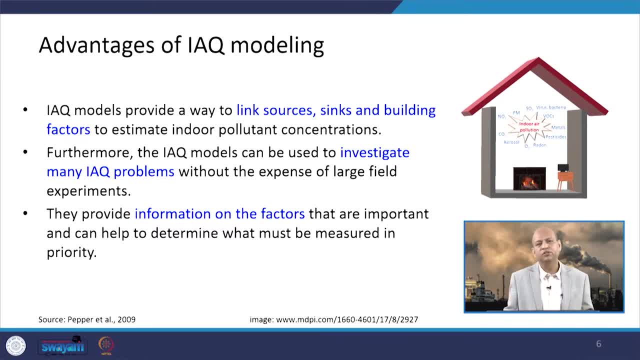 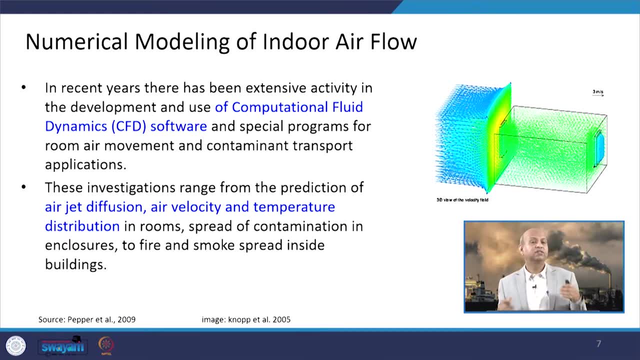 So those variable factors can easily be considered in the indoor environment, indoor air quality modeling When we talk about like numerical modeling of indoor air flow, because there are several techniques and one of those techniques is numerical modeling. In recent years basically extensive activities and research and development have been done. 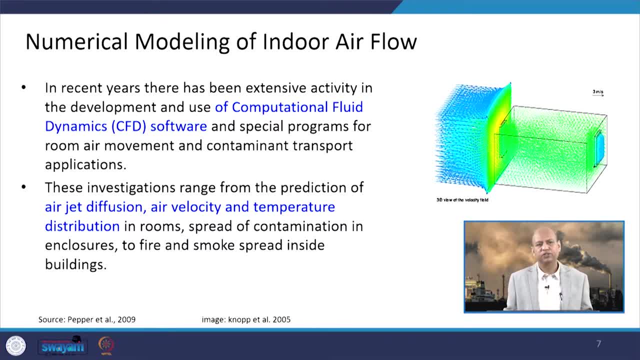 through computational fluid dynamic related processes, or software CFD which is called, which is you might have heard about this. So these are the special programs For like room air flow movement or contaminant transport applications within those indoor environment and these investigations they can range from, like prediction of air jet. 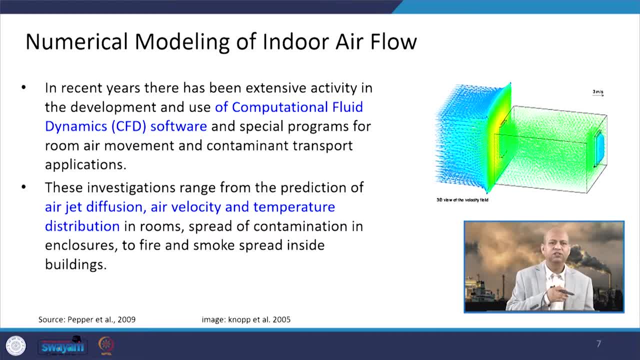 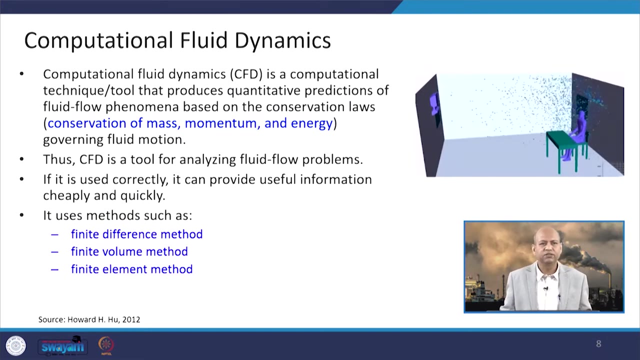 diffusion or air velocity or temperature distribution in the rooms or humidity related issues or contamination, diffusion, dispersion within those enclosures or any smoke spread inside the buildings. So all those kind of issues can be tackled by CFD techniques basically. So the CFD is a computational technique or tool, you can say, which produces quantitative 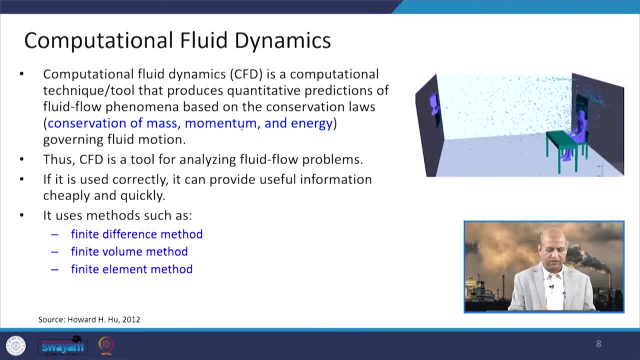 predictions of fluid flow, like through conservation laws, like conservation of mass, as I just said, or momentum, conservation of momentum, or conservation of energy. So those basic principles are used for this particular CFD technique, So they govern the flow, So they govern fluid motion, basically, 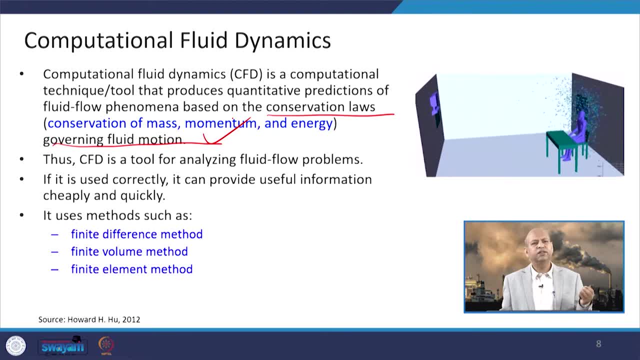 So these are the principles which are used. So you can say that CFD is a tool for analyzing air fluid or air flow problems And it is used, it can provide- when it is used correctly, then it can provide useful information very quickly and with minimum resources. basically, just you have computer. 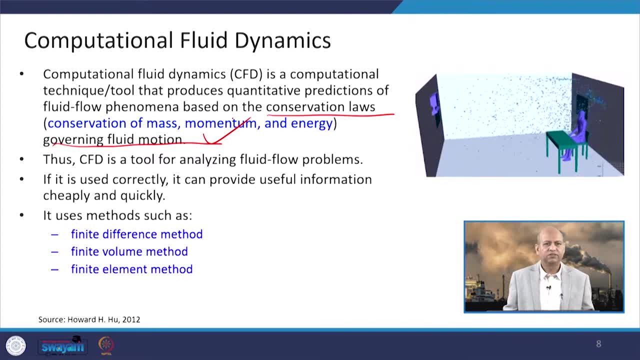 and you can run that model and you can get the results And it can use different methods or processes. So these are the principles which are used, So these are the procedures, like finite difference method or finite volume method or finite element method. 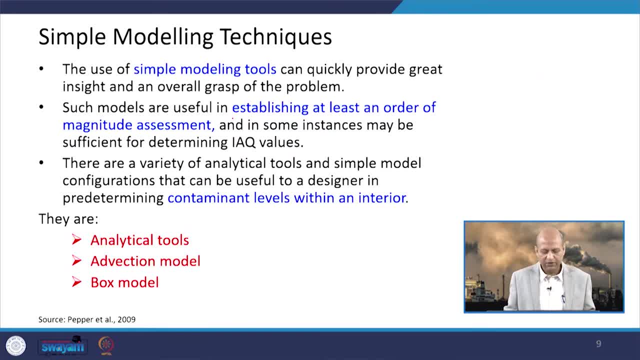 Those kind of popular techniques can be used for CFD models. Then there are other models which are of very simple nature. So these simple modeling techniques can also be used for indoor air quality modeling And they can be like related to analytical tools or advection model or box model. 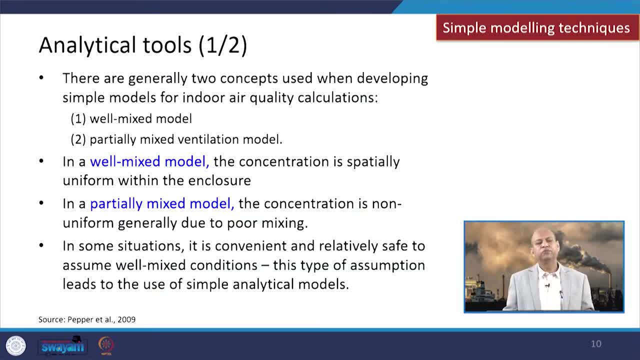 So we will see. what is those tools? Okay, When we talk about analytical tools, basically they are based on two concepts when we develop the simple models for indoor air quality calculations or estimations. So one is like well mixed model and other one is partially mixed ventilation model. 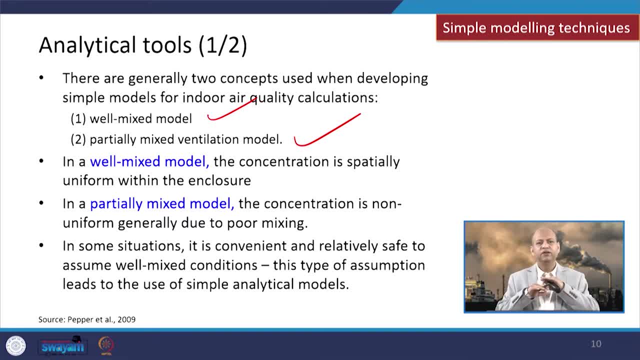 In well mixed model, basically we assume that concentration is uniformly distributed because it is mixed very well in that enclosure or in that indoor environment. In partially mixed model, basically, the concentration is non-uniform. It can vary from one point to another because of poor mixing or ventilation related issues. 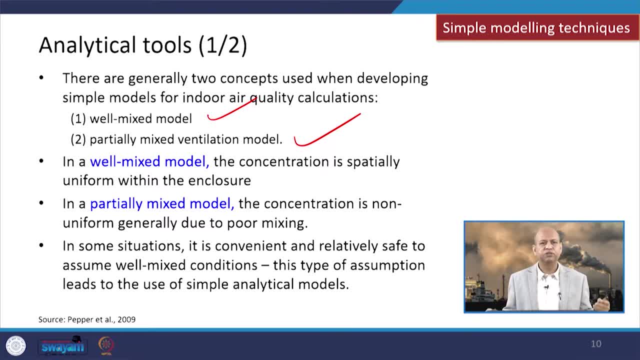 But in some situations there may be kind of mix of the things and it is relatively safe to assume well mixed conditions for simplification purpose, for approximation purpose, so that you can quickly calculate the needed parameters. So this type of assumptions can be used. 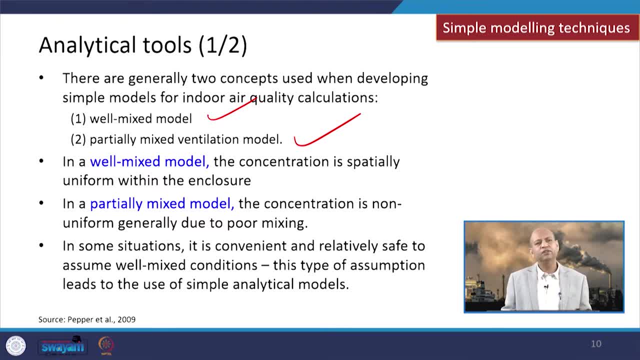 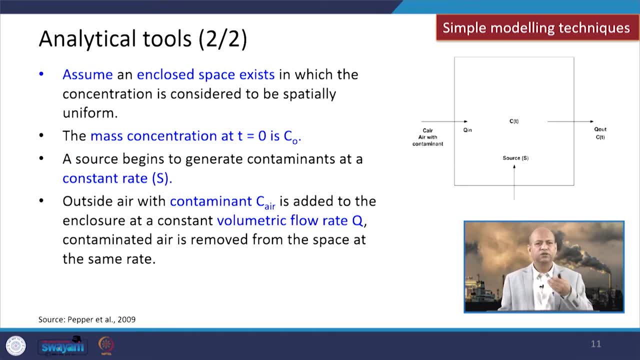 Okay, So this leads to the use of simple analytical models or tools. Further, there are certain assumptions, like we assume that an enclosure or that indoor environment exist in which the concentration is considered to be especially uniform. as I said, when we assume that it is uniform, then we assume that at each point the concentration 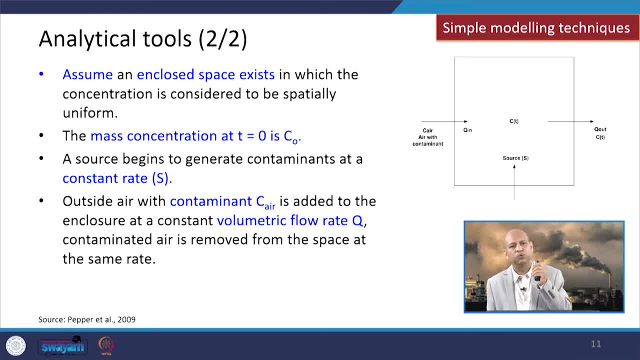 is same But the mass concentration: at time t0 it is c0, like then at the point, like at the time t it is ct. So maybe sea air which is the air with contaminant out outdoor air, if it is entering or not only. 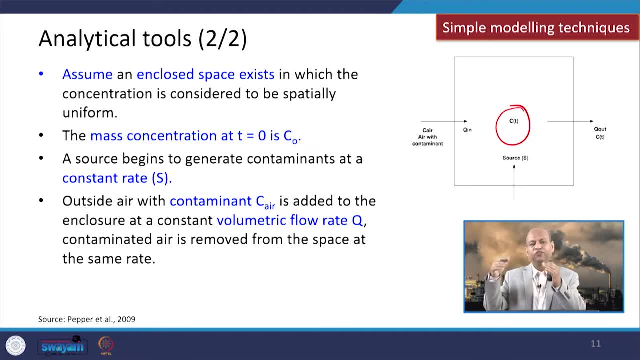 in the outdoor but within the indoor environment also, if we are assuming certain cubes or certain small enclosures, So from one enclosure to another air movement may be there. So this sea air which is with certain contaminant if it is entering into this particular enclosure. 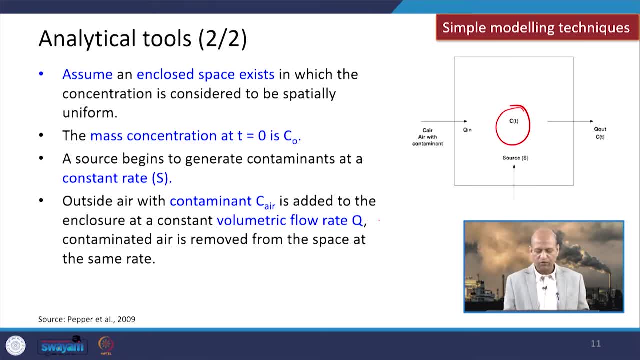 then it can have this: Okay, So volumetric flow rate q in and the concentration it can have c in or at the time t0. if we assume c0, then at time t the concentration may be ct and that ct can be like sea air when it. 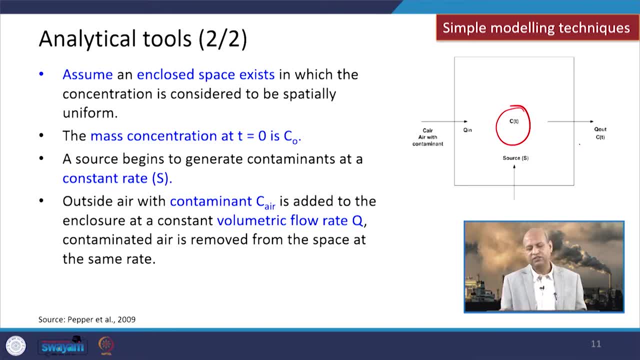 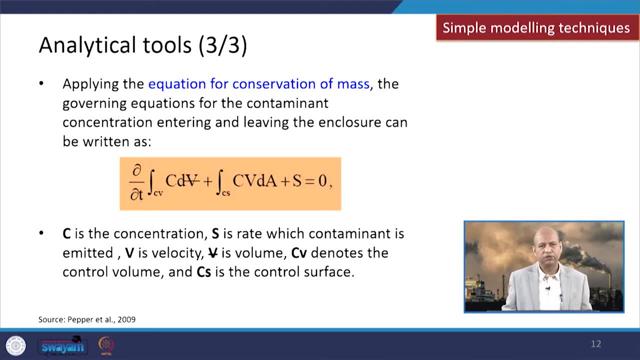 is uniformly distributed in this enclosure and that same concentration will go out, because every corner, every point has the uniform concentration in that particular space. When we talk about So there are several like equations. there are several equations, but for the sake of information I give you this very only one: conservation of mass related equation, which 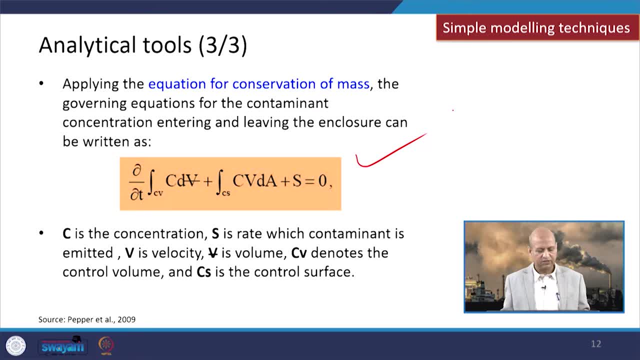 is used for estimating the concentrations and solving this, these equations. So where these parameters are concentration, then this contaminant rate which is being emitted, v is the velocity, and then this volumetric parameter is there, then control volumes factor can be there And control surface related factor can be there. 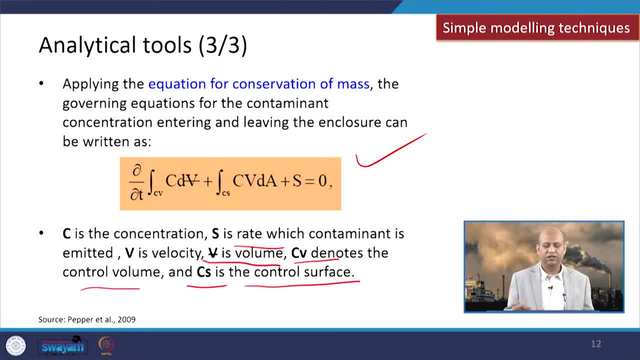 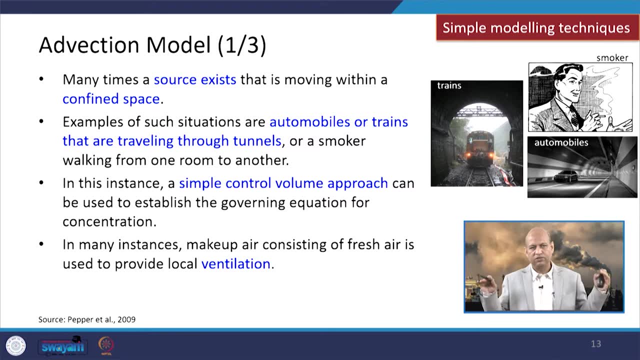 So these equations are solved by the model and they can estimate the concentrations ultimately. Well then, other model is advection model. advection, you know horizontal movement, as you know, convection is vertical movement. advection is horizontal movement In many times like source exist that is moving within a confined space, like in a tunnel train. 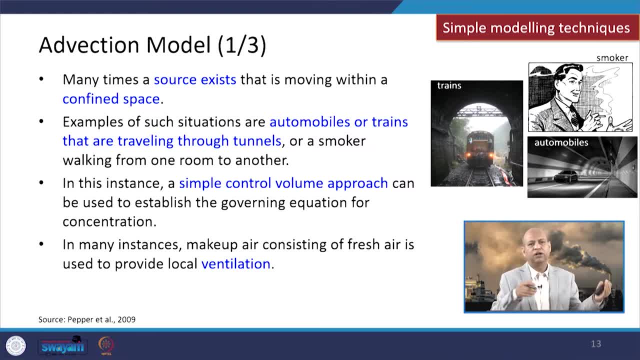 is moving, Okay, Or within the you know household activities, Okay, Okay. So all these people are doing and they are also moving, like somebody is smoking and moving in the corridor, So those kind of moving sources may exist. so it is a horizontal movement. 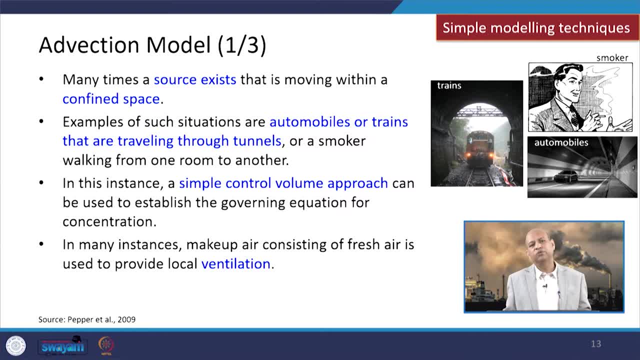 So advection models are used to, you know, simulate or model the effect of those sources and to know what would be the concentration at the point of interest. So we see all those parameters, of course, like volume approach is used, control volume approach is used. 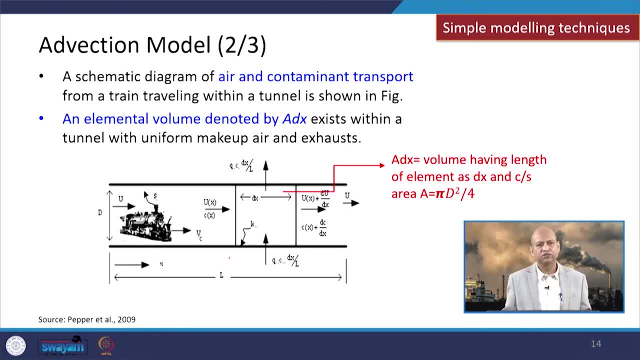 And then these ventilation related parameters are also used. You can see in this particular figure it is shown very nicely that you know this. adx is volume having length of element as dx. you know this much of slice of the dx and area is. you can have this area of this tunnel where this engine or train is moving, u is the velocity. 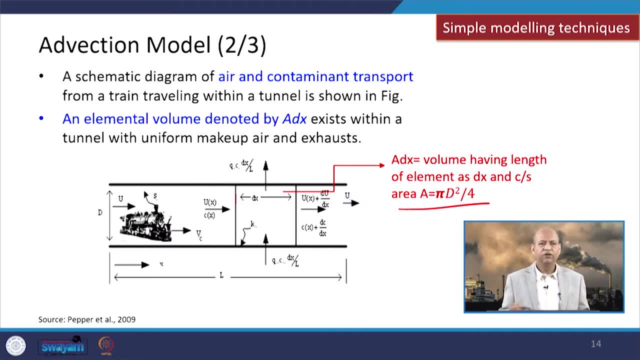 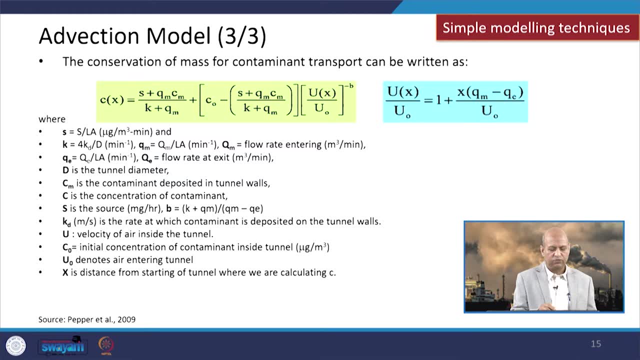 So you can use those equations. Okay, So you can further solve it to get the concentration. Then advection model uses all kind of you know those equations, but ultimately this is the final equation which is used for estimating the concentrations where different parameters 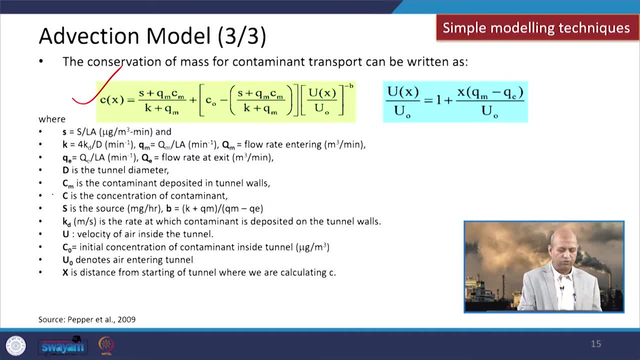 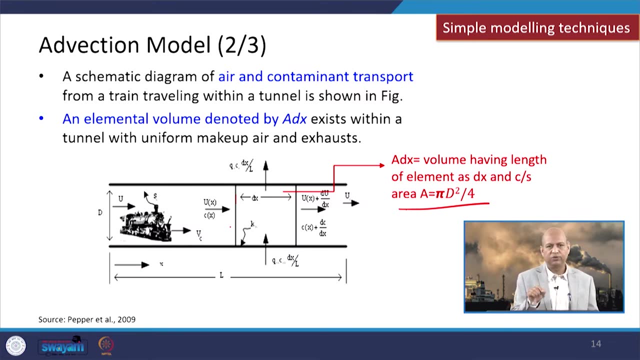 are there, like contaminant deposited in tunnel walls. cm c is the concentration of the contaminant, which is, you know, like cx at the x distance. you can see here. this is the, you know, this l is the length of the tunnel. Okay, So wherever point you are, you know denoting the x distance. so that is used in this equation. 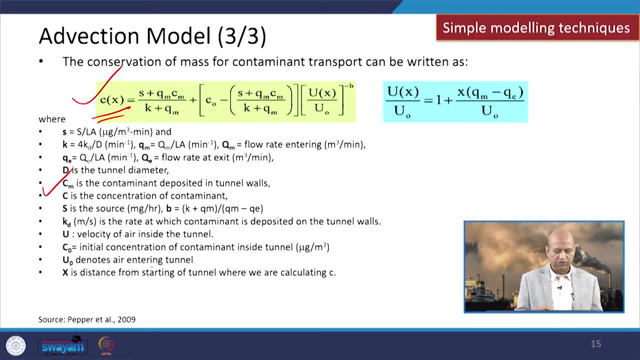 Then u is the velocity of air inside the tunnel. u0 denotes the air at the entrance of the tunnel. basically, x is the distance from a starting of tunnel at the point where we want to estimate the concentration. So all these parameters are basically used to estimate the concentration through the 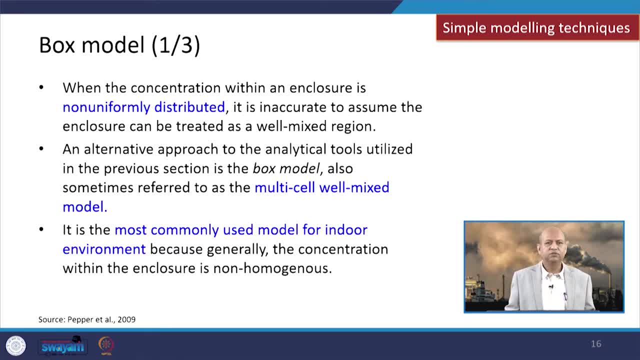 advection model. Next is the box model and this box model is basically, you know, This box model is used when non-uniform conditions are there, when concentration is existing in a non-uniform way, which is a reality. basically Uniform concentration we assume in certain enclosures, but if larger, you know enclosures. 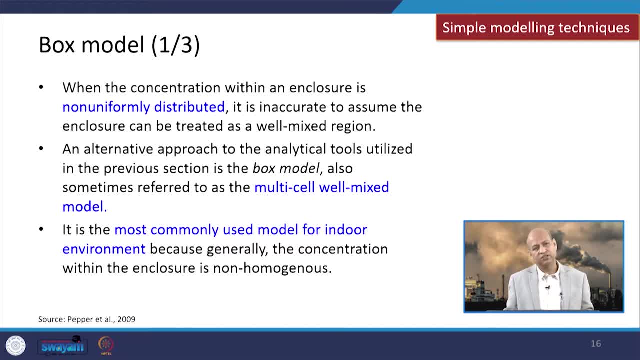 or indoor environment is there, it is not necessary that uniform concentration will be there of a particular pollutant. So basically, box model is based on multi-cell. well-mixed model means small cells are like. if this is the box model creating, so it can be divided into several cells and those cells 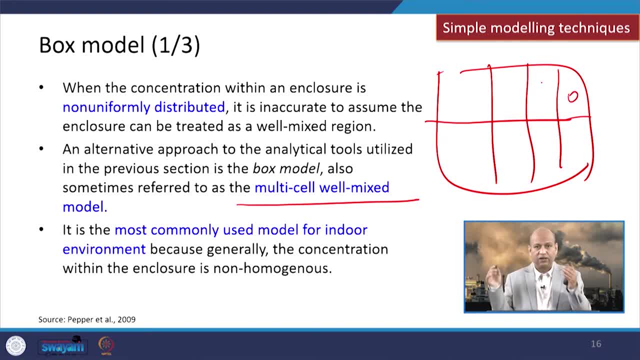 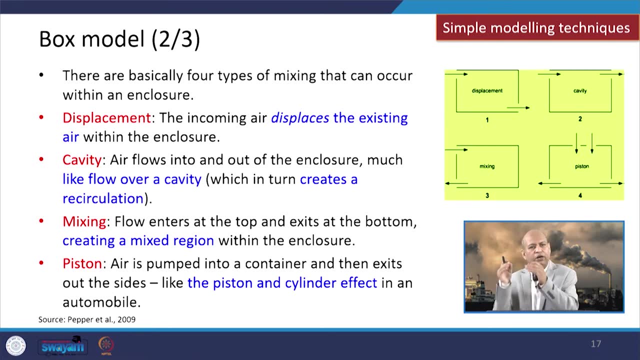 can have different concentration of uniform level, So each cell can be termed as a uniform concentration related phenomena and then integration can be done at later stage. So basically, non-uniform condition is existing, but that non-uniform condition can be divided into several uniform cells. 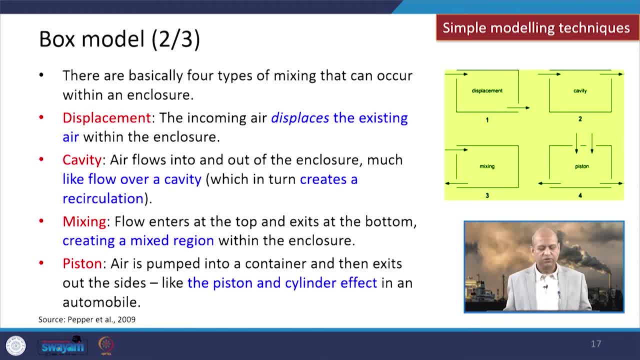 Right, So, and this box model, basically, you know, have four types of mixing which can occur in those cells which we have divided, for example, displacement. So let us say, if air is entering in that way and you know it is coming and going outside, 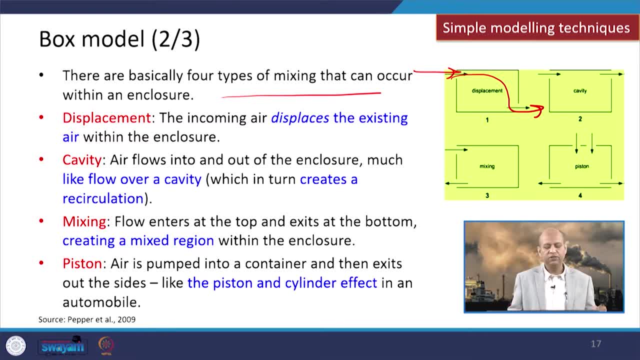 this way. So it is displacing basically. So incoming air displaces the existing air which is in the enclosure or in the cell. it goes out and then cavity formation can be there, Like it is there, like air is coming and it is going directly. 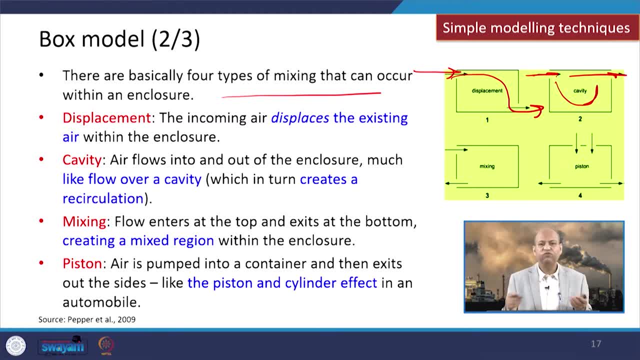 So here, this is the cavity. So this cavity can form and concentration may build up rather than flushing it out. In displacement kind of phenomena the flushing of concentration of pollutants may be there, but in this kind of condition or context the cavity formation can be there and concentration. 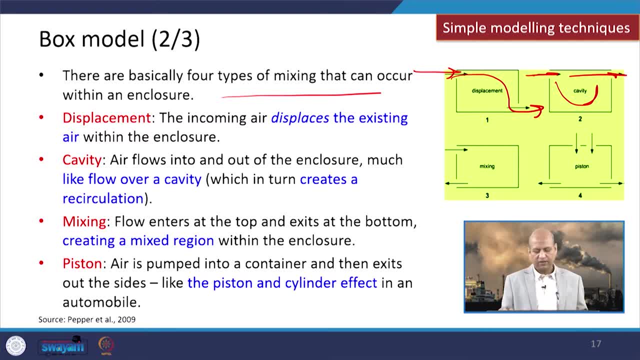 build up can be over the period of time can be there and recirculation of concentration may be there, Right? So then there is this mixing, like if this air goes and travels a long distance and come back, So kind of mixing region or mixed region is produced and uniform concentration you. 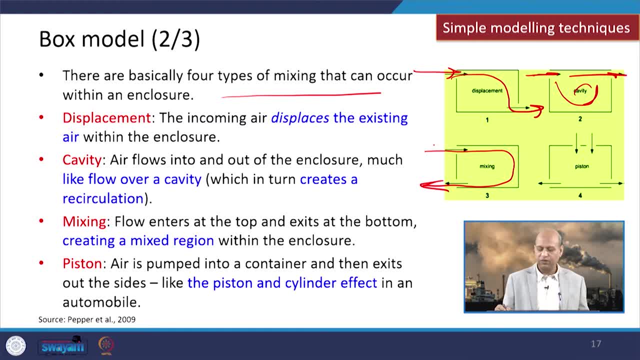 can assume, in this particular cell. Then there may be another way, like piston, where air is coming from this and air is going out of this. So it is working like a piston and it is pushing out this air outside. so several kind of combinations can be there which can be catalyzed. 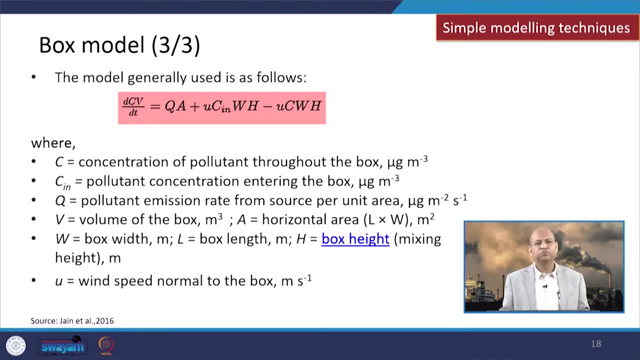 Right, So this can be catalyzed or simulated by box model, basically, And this is the fundamental equation which is used for estimating concentrations, based on several parameters like pollution, emission rate, and then the area, this horizontal area length into width, and you can have this, as is the box height. 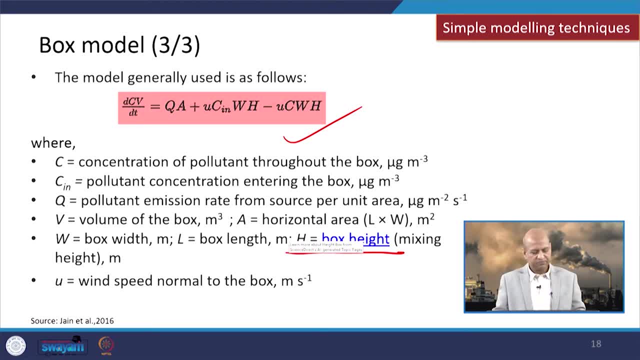 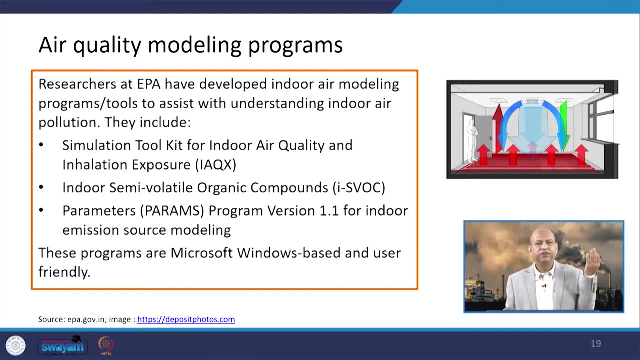 So box height basically, when we are talking about the mixing height within that enclosure, Okay, Mixing height in ambient air is boundary layer height, but within the enclosure or within the indoor environment it can be again the some mixing height basically. But fundamental concept is same. we use box model in ambient air quality modeling also. 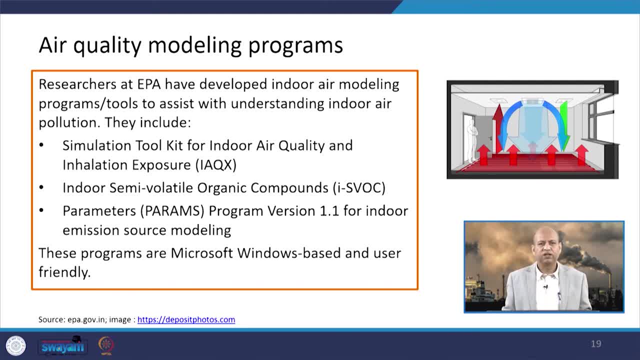 Right. Then we come to air quality modeling programs, which are like readymade tools available, because US EPA, Environmental Protection Agency, has developed certain tools which can be used by people to So they can simulate air in different indoor environment, and they can get easily those. 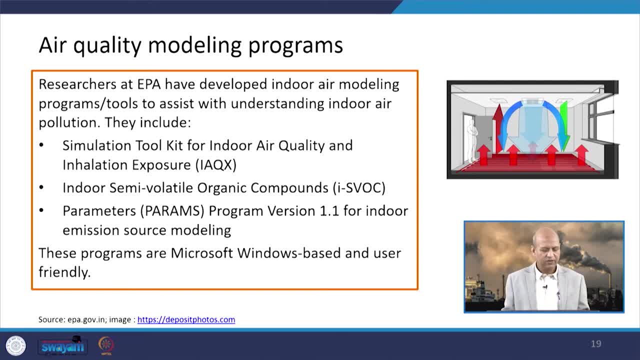 models are handled or those programs are handled So like. one program is simulation toolkit for indoor air quality and inhalation exposure- IAQX. Another one is indoor semi volatile organic compounds, IASVOC. Then third one is parameters or PARAMS program, version 1.1.. 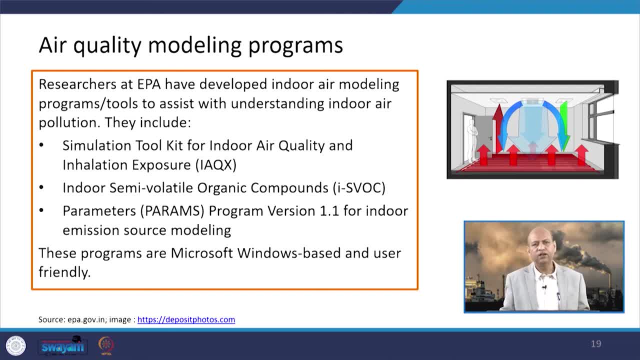 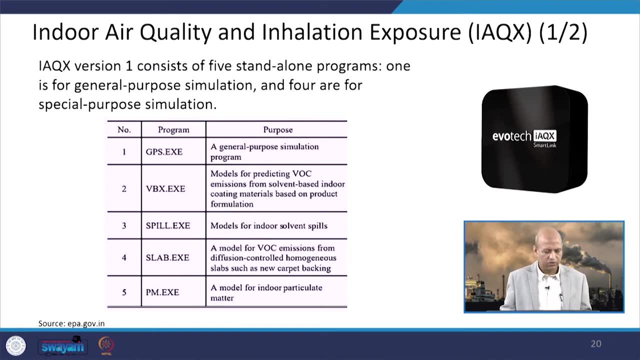 It was earlier 1.0, as we discussed. Okay, And this four indoor emission source modeling basically. So these programs are window based, so user friendly and anybody who knows simple computer handling. they can easily use those tools or models In indoor air quality and inhalation exposure, like IAQX model. basically, there are different. 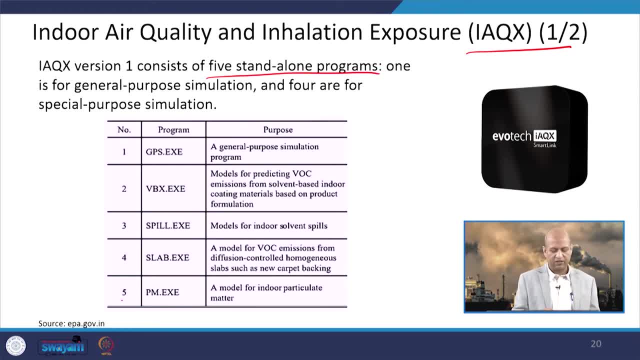 standalone programs or modules, like five modules are there, One is like GPS, So this: Okay, So this file can be executed, or this program or this module can be executed for the purpose of general purpose simulation program, basically When this VBX is related to VOCs, so it models to predict the VOC emissions from solvent based. 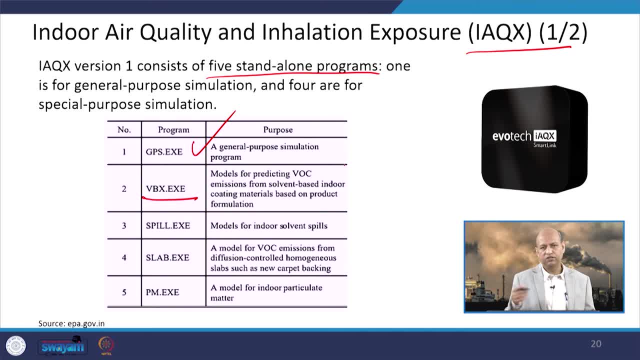 indoor coating materials based on product formulation. This may be like furniture, this may be from walls, etcetera. then spill this spill related module is there which simulate the Okay, Which models for indoor solvent spills where some solvent has been spilled out, then it. 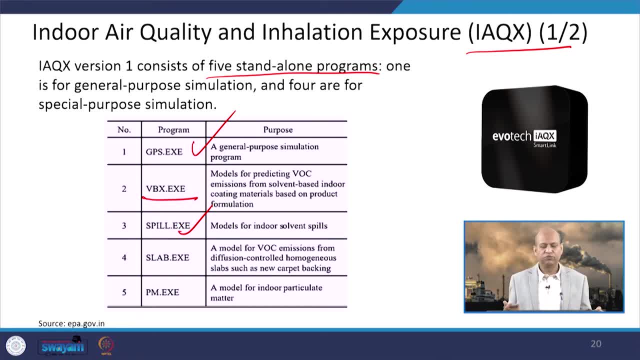 can be modelled because it will give some VOCs, etcetera. or then this is slab, So this model gives the VOC emissions from diffusion controlled, homogeneous slab such as new carpet backing. So if carpet is there, new carpet is there, lot of fumes may be there. so this particular 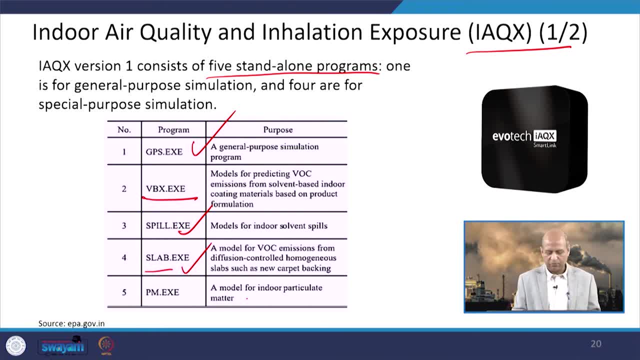 module can be used for that particular emissions. A model for indoor particulate matter is PM related module. So if we want to run a particular module depending upon the requirement, we can run. otherwise we can run five modules if all these conditions are applicable. 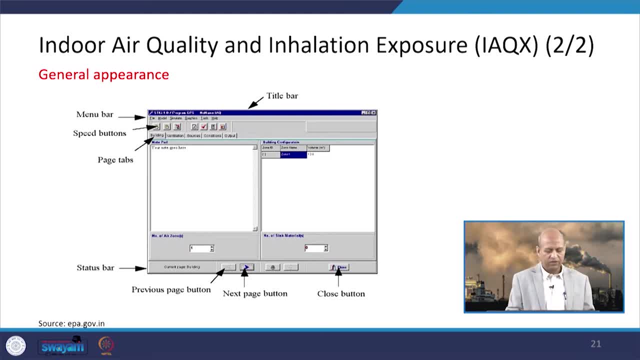 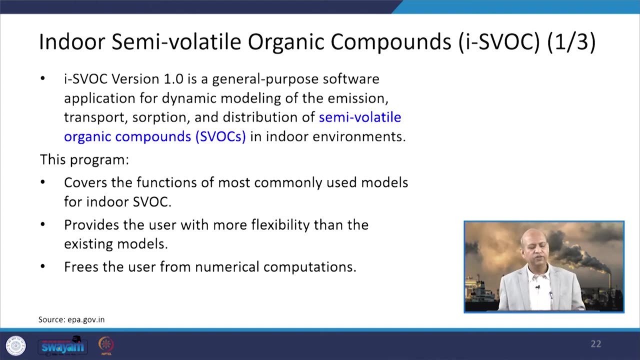 You can see, this is the general appearance of that particular tool. so different buttons are there and because it is window based, you can just press the button. you can go through the menu bar. Okay, You can see whatever possibilities are there. So, basically, the next one is indoor semi-volatile organic compounds- I-SUVOC. 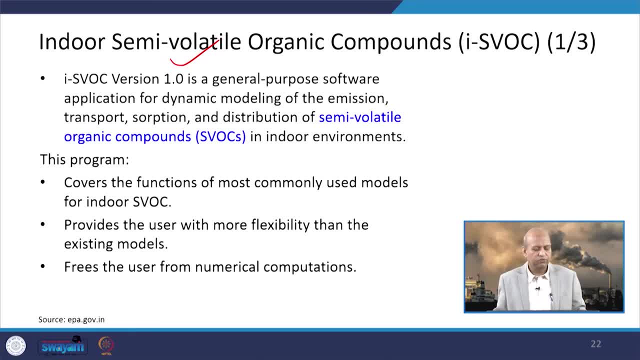 Okay, So this is 1.0. I-SUVOC version is there and this basically model the emissions and the its transportation or absorption, or adsorption and distribution or dispersion of semi-volatile organic compounds, SVOCs, in the indoor environment, and this program is capable of covering the. 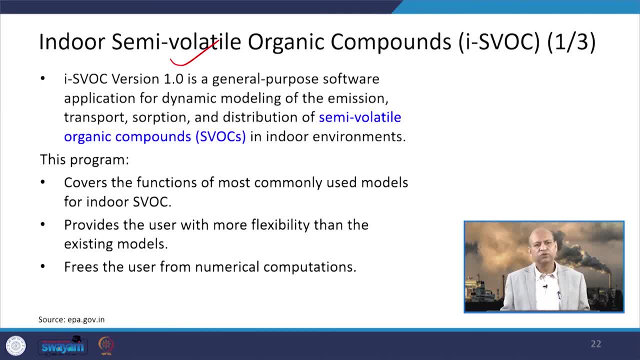 functions of most commonly used models. Okay, So it can also provide the user with more flexibility than the other existing models. So that way it is versatile, you can say, and it frees the user from numerical computations which are quite resource intensive as well as it needs lot of skilled manpower. 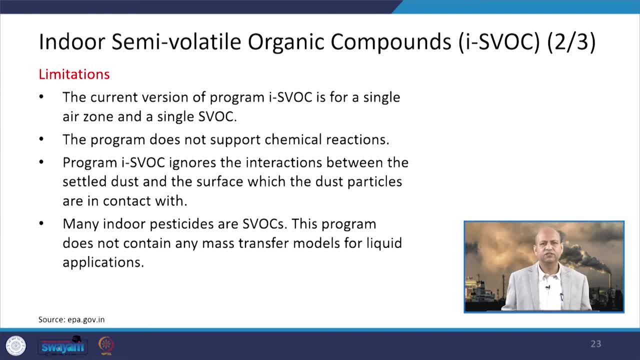 So that way it is quite easy to handle and it has versatility. but there are certain limitations also. Okay, So the current version of this program is for a single air zone and a single semi-volatile organic compound, So it cannot model the mixture of different kind of VOCs. 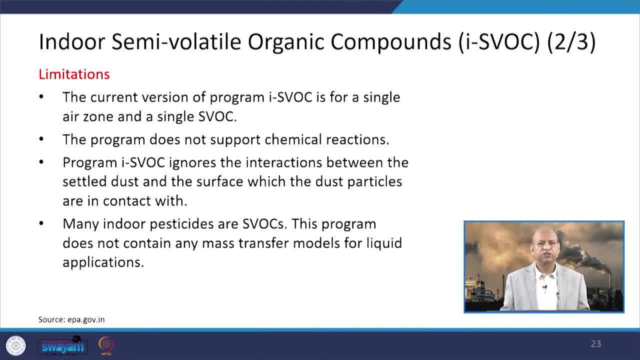 The program does not support chemical reactions. so that way, very simplified assumption is there. This program ignores the interactions between settled dust and the surface which the dust particles are in contact with. Okay, So the indoor pesticides are there which emit SVOCs. so this program does not contain. 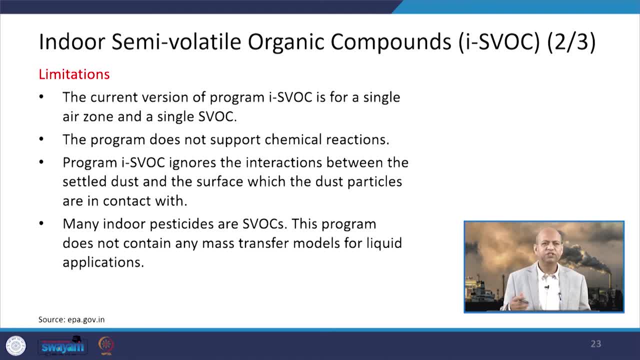 any mass transfer models for liquid applications. So these are limitations, but, as even in Gaussian dispersion model, when we talked about in ambient air quality modeling, there were several assumptions, so that because there are so many uncertainties and complex things are there, we cannot handle everything otherwise. 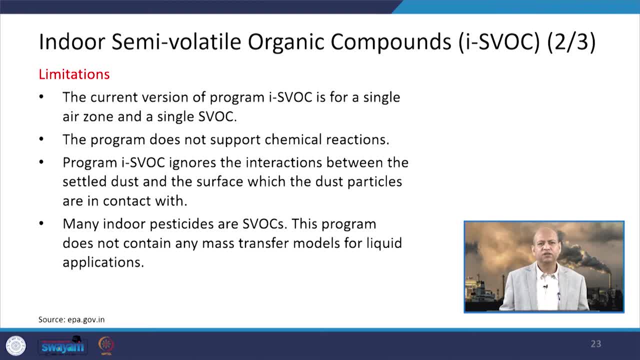 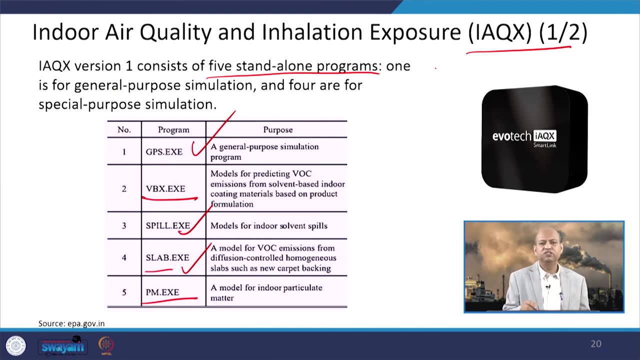 the model will be very complex and very difficult to handle. So that is one of the limitations. Okay, So it is fine if there are certain limitations, but if it is given good results. but other like in this particular model we had these five modules, so that way this is better model. 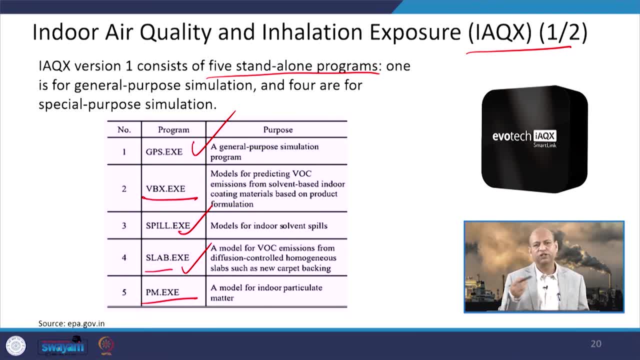 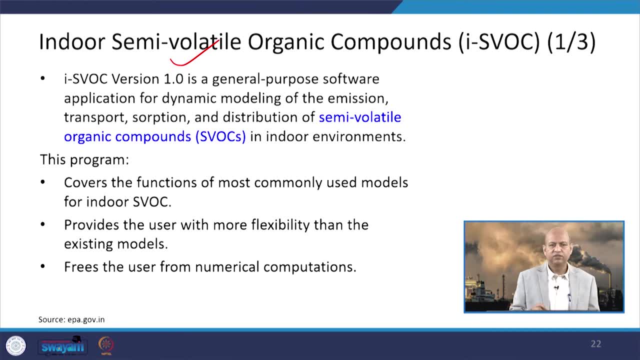 if you want to model several kind of VOCs, particulate matters or spillover related issues, but if you want to concentrate only on semi-volatile organic compound, then this model is fine. but only limitations are there that because it handles single SVOC atoms. 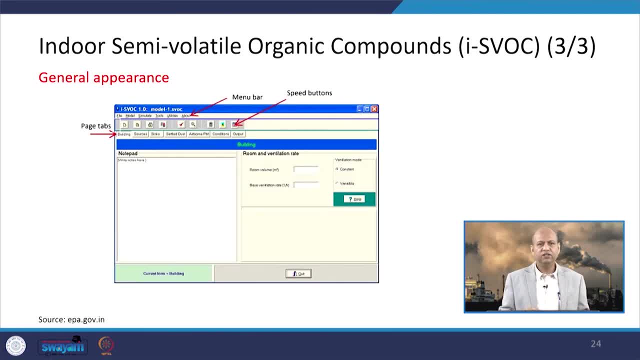 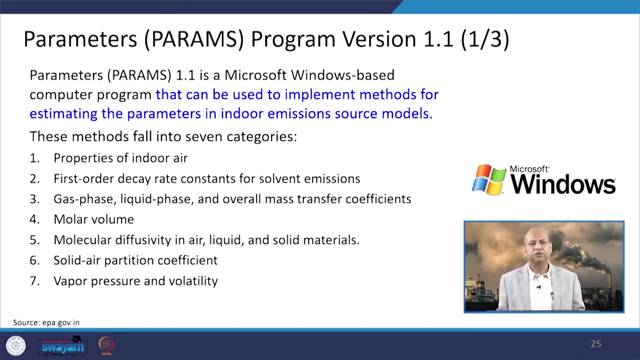 Okay, So it is fine. if you see at a time then it can be seen this general appearance, again similar to other one window based model it is. so you can just use these buttons and you can run the model. The third one is parameters- PARAMS program version, which is of 1.1, ISOVOC was of 1.0. 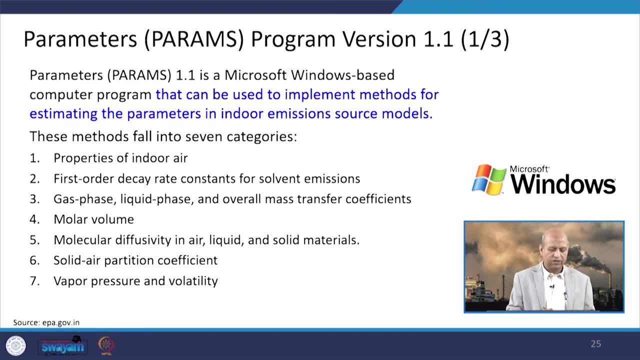 and this is 1.1,. well, so these, this particularly program, can be used to implement mass transfer methods for estimating the parameters in indoor emission source models. that is why it is known as PARAMETERS, PARAM 1.1.. And the methods, which fall in seven categories, which are used in this particular program. 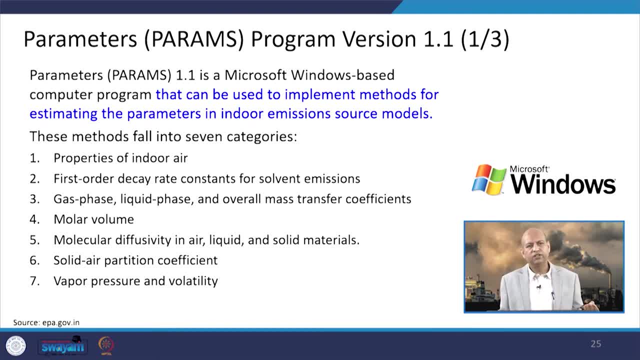 or tool are like properties of the indoor air. first order decay rate constraints for several emissions can easily be handled. then gas phase, liquid phase or overall mass transfer. these parameters, So these coefficients, can also be taken into account. molar volume related parameters. 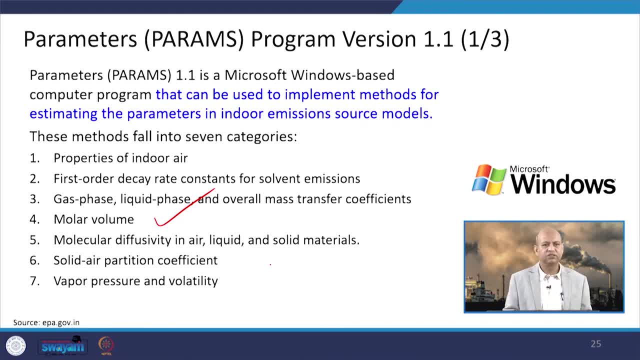 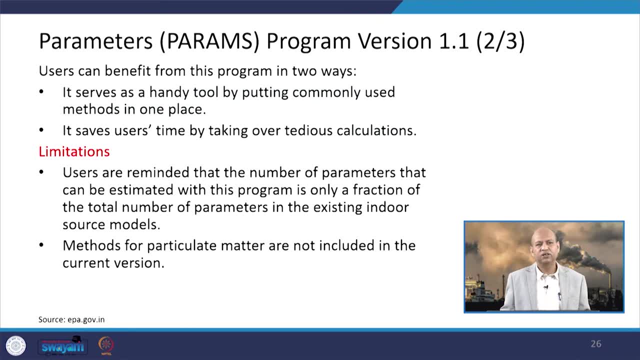 then molecular diffusivity in air, liquid or solid materials, solid air partition coefficients, vapor pressure and this volatility- all these things are taken into account with this software. Then users can benefit from this program in base two fundamental ways. this can serve. 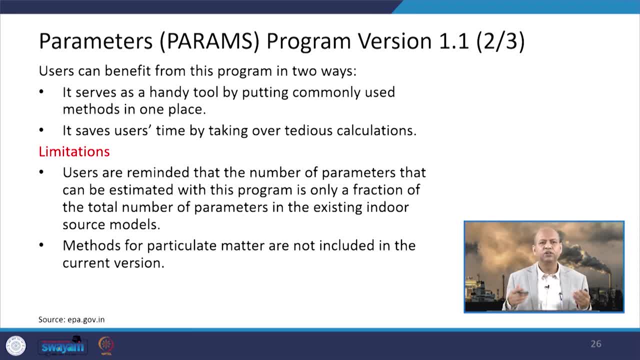 as a handy tool by putting commonly used methods in one place, And it can save a lot of time because tedious calculations are avoided. this program does all those calculations at the back end, but there are limitations. again, like earlier model also had limitations, this users are reminded that the number of parameters that can be 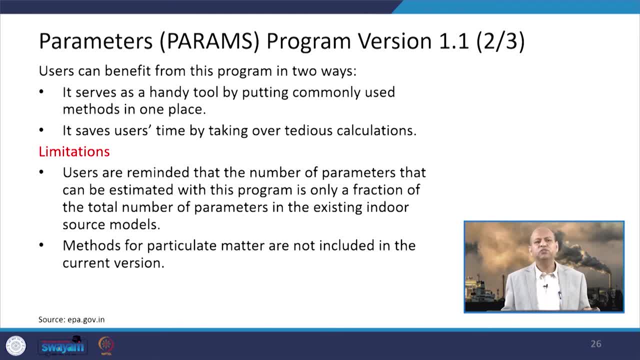 estimated with this particular tool is only a fraction of the total number of parameters in the existing indoor source models, So not all parameters are being handled, But important parameters are being included, And these methods for particulate matter are not included in the current version. 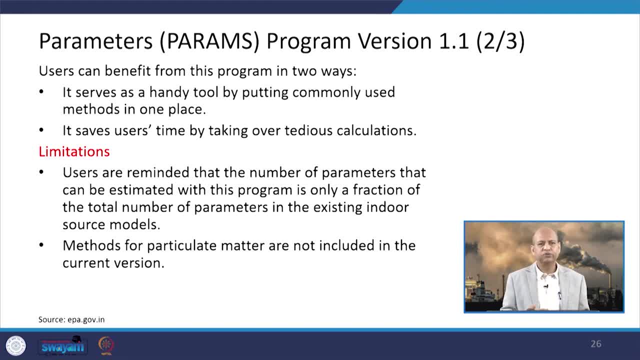 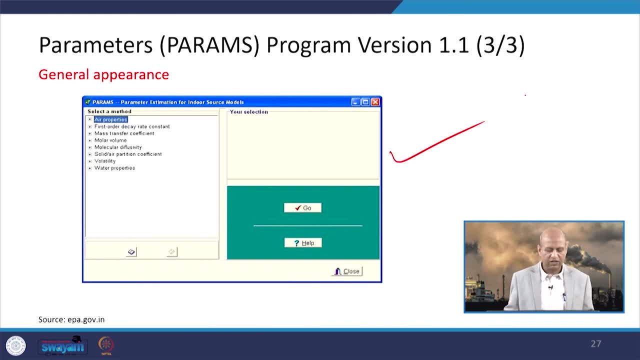 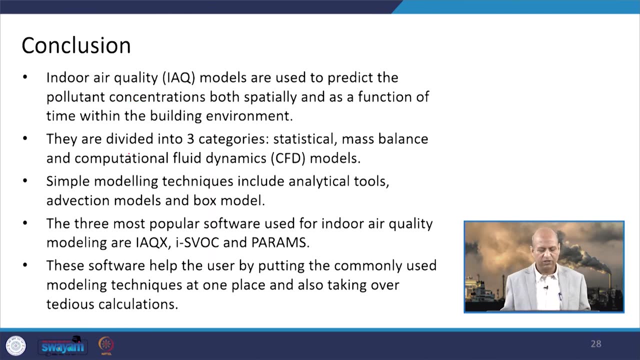 So that is one limitation. It can have other pollutants but particulate matter related. if you want to model, then go for that. Iaqx, that is fine. This is the general appearance. again, all these selected methods are given. So anything you can choose as per the requirement and you can run the model. 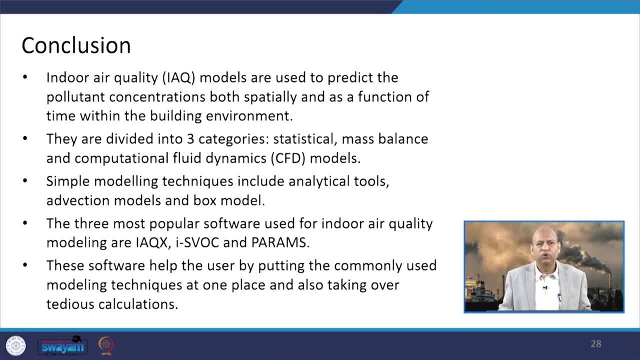 So, in conclusion, we can say that the indoor air quality is very good, Thank you. So, as I said, the indoor air quality models are very important for predicting the pollutant concentrations, in terms of especially like from one point to another or as a function.